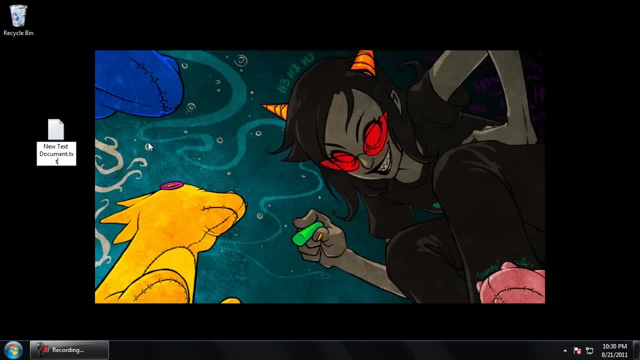 to start with a text document, and this is assuming you have the show extensions box unchecked. I'll put a little description, a description or a link on how to get the the extension. I'll put the extensions for files set up in the description, but pretty much turn off that little. 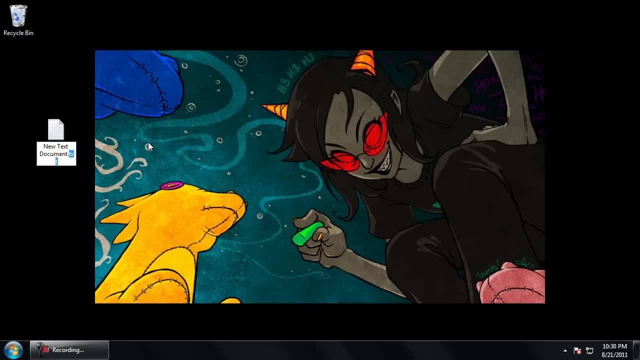 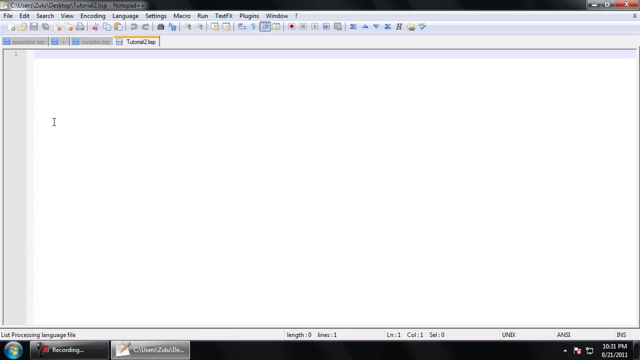 checkbox, because that is the great evil of the world. So for the extension here, I'm just going to give it dot lisp for the name. I'm going to give it tutorial two. So open that file up in whatever text editor you like. I like to use notepad plus plus because it gives me a nice 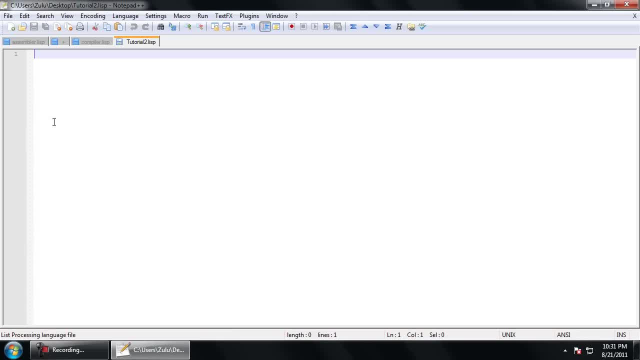 little syntax highlighting with Lisp, and it also matches parentheses and things without me having to, you know, install anything. So what we're going to go ahead and do is first examine the syntax of a proper Lisp program. A Lisp program consists of zero or more, that's right- zero- forms. A form is either an atom or it's a list. 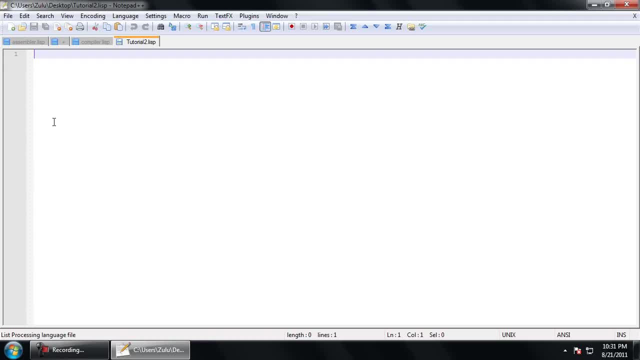 Now, atom is any of the sort that you've seen already, which is such as an integer, a floating point, number, a character. Additionally, a couple of more. atoms are, for example, the string, which is open quotation, then a series of characters such as hello there. 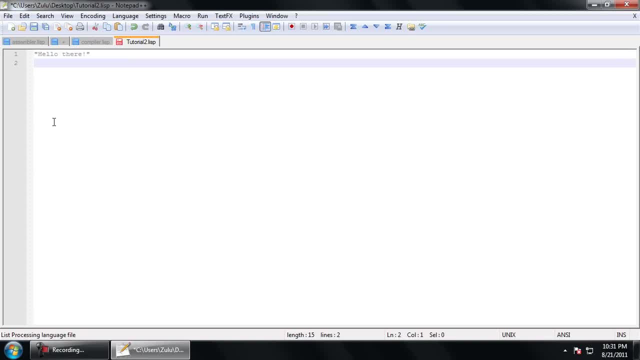 Another. another atom would be very, very similarly related is the vector, which is a, which is a single dimensional array which contains any elements that you'd like In in Lisp. Lisp is a dynamically typed language. This means that there is no forced declaration of types. 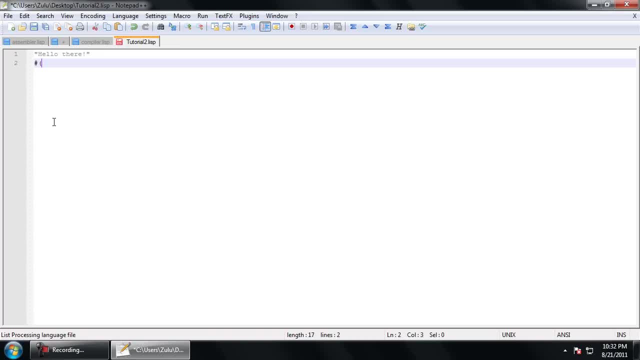 You can. you can declare variables and other things to be of specific types in order to optimize your program, but it is not strictly necessary to do so. And that's relevant for vectors, because vectors can hold elements of any data type. So here we can have zero one and then the string hi, and then we can have 10.3.. 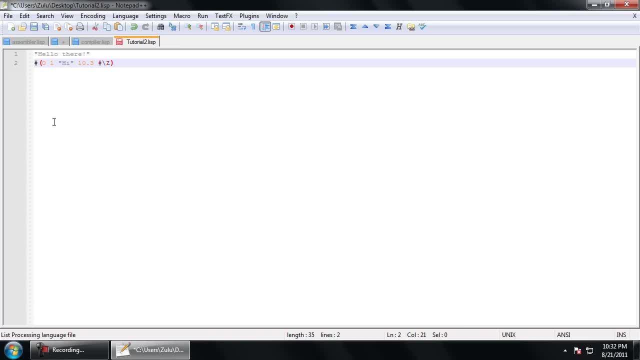 And with the character z, because I like z, And that is a valid vector. A vector starts with a pound sign followed by an opening parentheses, and then you have your, your list of your list of elements. in this case would be zero space, one, etc. 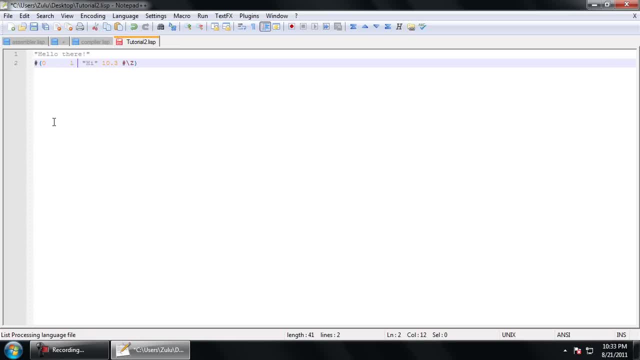 The space is necessary just to separate elements, but you can have as many spaces as you'd like, such as in this monstrosity, And then, when you're done typing elements, you go ahead and close out the the that list with the closing parentheses. 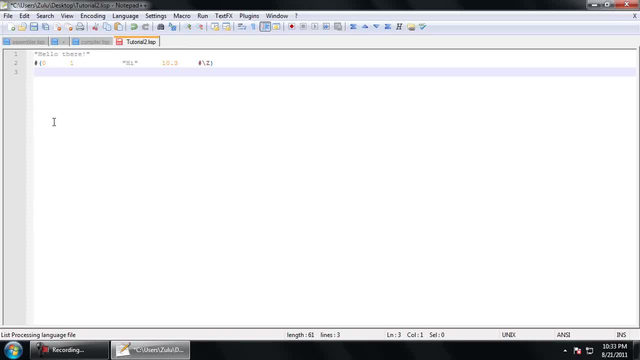 And speaking of lists, the Lisp stands for list processing, in case you didn't know. So lists are actually very important in in Lisp, A list program is actually just a list of lists Upon lists, And that's because, as I said, a list program consists of either: 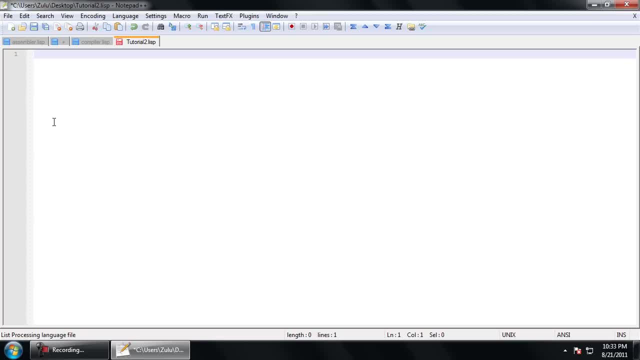 of multiple forms, which are either atoms or lists. So let's examine lists. Lists are created by having an open parentheses, then a series of values. Again, you can have an empty list, which is also equal to nil. We'll go over that in a second. 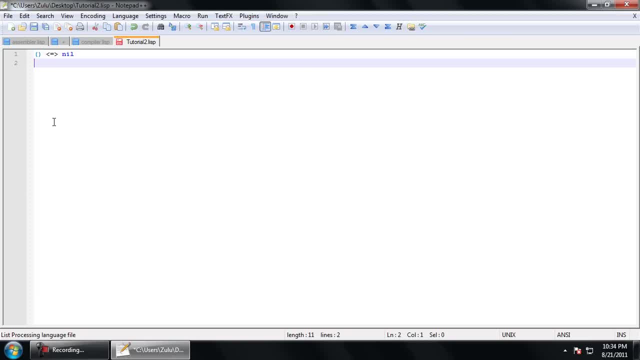 Let's use that instead. And we can also have a list of one or more elements. So say this would, for example, would be the list that contains zero, one and two. So the way a list is evaluated, atoms are evaluated essentially to themselves. 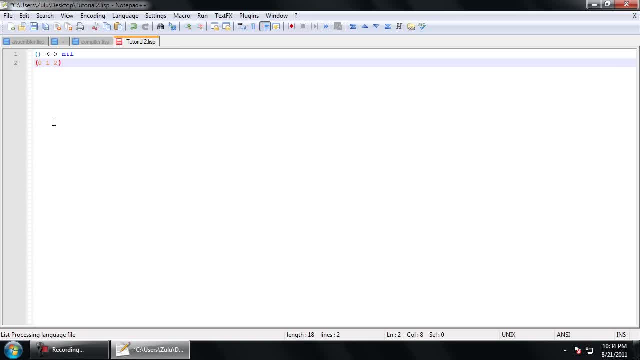 That's kind of a misnomer, but we'll get to that eventually. The way lists are evaluated, however, is that their first argument is kind of special. The first argument stands for the name of the function defined in the system currently. 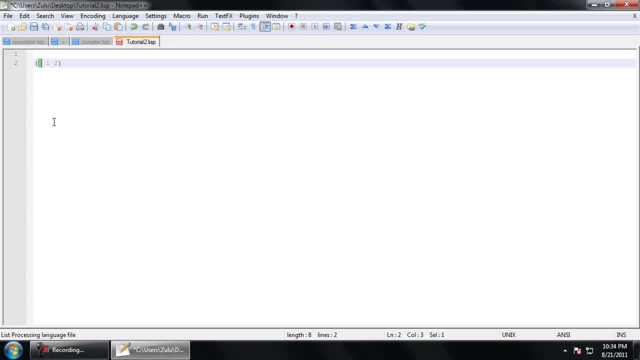 What it's going to do is it's going to invoke that function by evaluating each of the elements left or right. So here are, first to last, because we can go ahead and introduce, for example, new lines and things like that. This is still the same list. 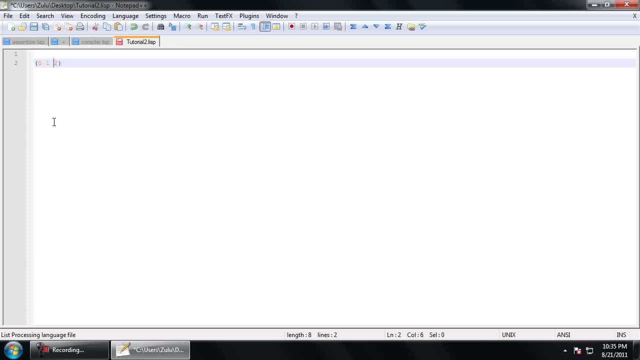 So it's going to evaluate the one, It's going to evaluate the two, And then it's going to evaluate, And then it's going to get the function called zero and call it with these arguments: Now there is no function called zero. 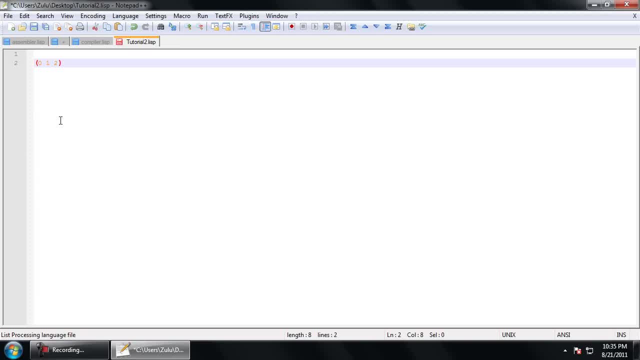 You can go ahead and make one, though because zero is a singular digit, you'd have to use a little special syntax for that. But anyway, let's go on and let's set up a correct function call. So let's do princ and give it the string hello world. 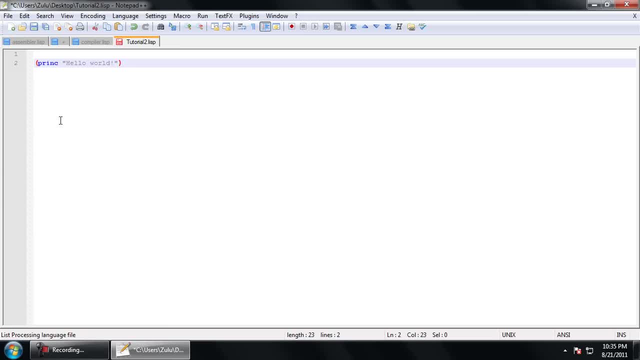 Now the princ function is going to take a lisp object. in this case we're giving it the hello world string and it's going to print it out to standard output in a way that's pretty to the user. So this is going to be our very first program. 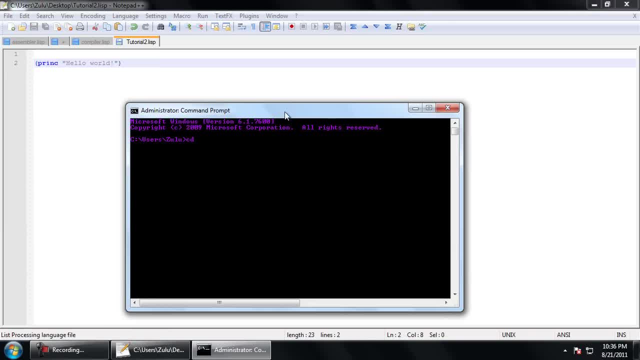 Let's open up command prompt. Navigate to the correct directory. Mine is on the desktop so I can go see users zulu desktop. or, since I was already in the zulu directory, I can just cd into the desktop cd being change directory. 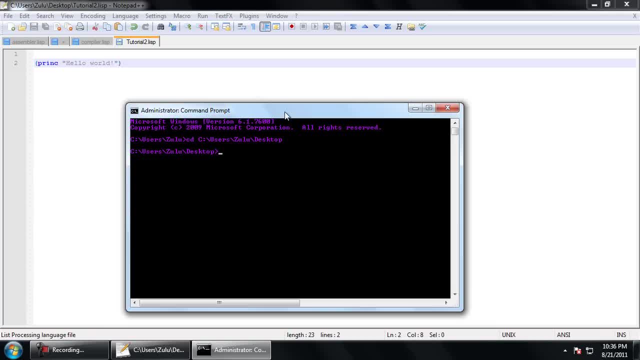 In this course. hopefully you'll be a little more accustomed to command line. So, anyway, we go ahead. now that we're in this directory, open up SBCL And we're going to use the load function. The load function is going to take as its first argument the name or path of a file. 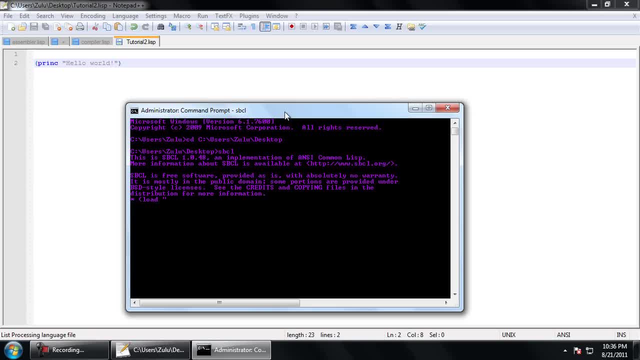 For now, we're just going to be using the name as a string of a file. It's going to open up that file, evaluate each of the forms in that file, top to bottom, and then it's going to tell us whether it was successful or not. 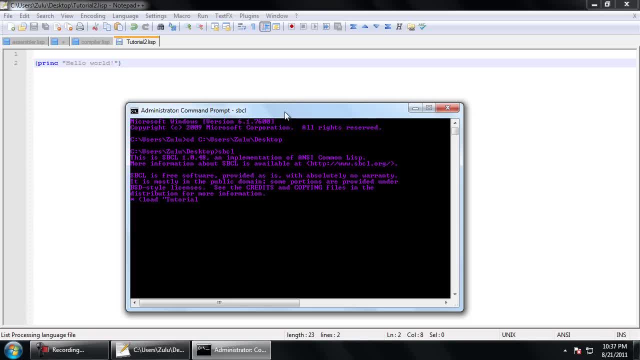 So here we're going to give it the name of the file as a string tutorial. So let's go back to that Lisp and go. As we can see, here we have hello world because of the printc function call that we made here. 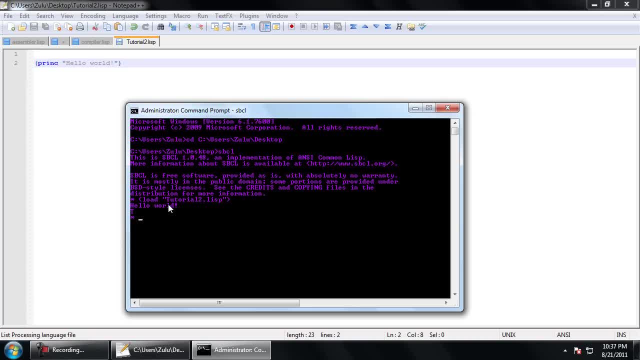 And then we have t Remember that we are still in the REPL. so this t is actually coming from. this t is actually the value of load. It's just telling us t for successful. In Lisp We have t true and false, represented by T and nil. 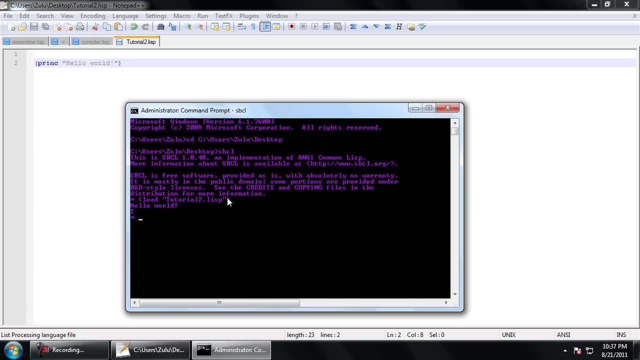 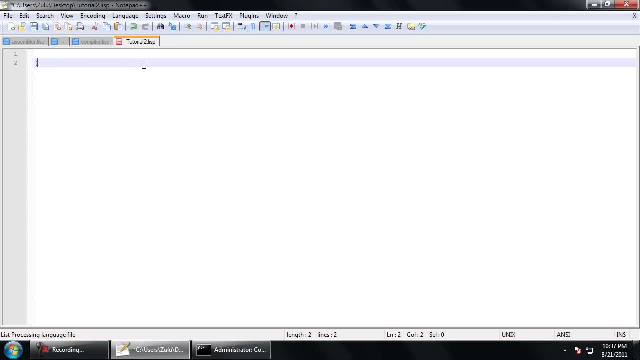 though, as we'll see in a second T is not the only truth value. actually, anything that is not nil means true. so in dealing with true and false, let's make a program that makes a decision. so here we're going to learn about the if special operator, the reason, the, 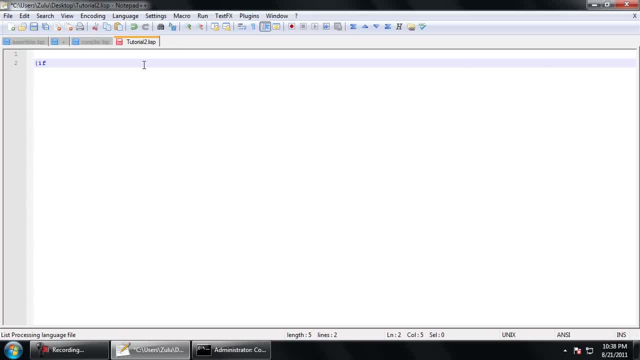 an if is a special operator and is not a function. it looks like a function call but it's not. is because if does not necessarily evaluate all its arguments. as I said before, a function will go ahead and evaluate each of its arguments left or right, every single one of them, and then it's going to 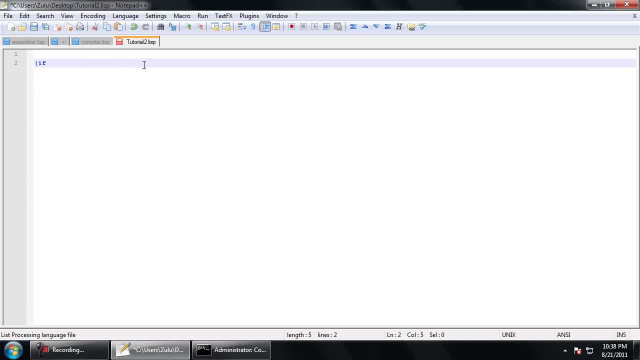 call the function that you name. with those arguments, however, a special operator is allowed to not evaluate certain what, what, what certain pieces of the, the arguments. if we'll go ahead and take as its first argument a condition, a, an expression that evaluates to either true or false, 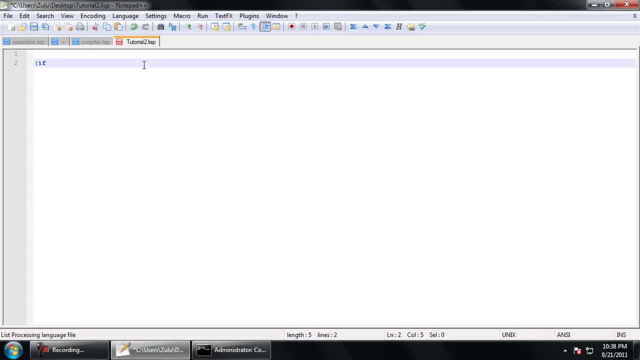 and it's going to do something based on that. so here we're just gonna keep it simple and just give it T for true. uppercase or lowercase does not matter, for symbols, same for the function. here we can type if, and all uppercase to say that we're serious with this. 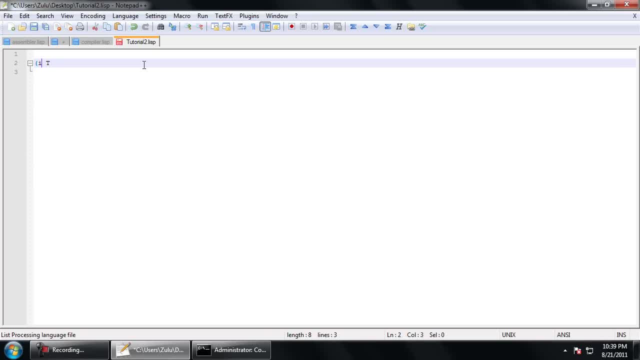 nobody does that, though also, let's be nice to lisp. so if T, we're going to do something. so here let's say princ hello or yes- yes is better- and here we're going to have princ no and let's close the if form. so what's going to happen here is that if 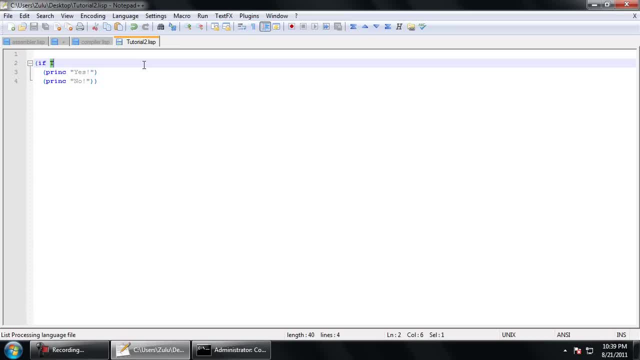 we'll evaluate the very first argument, in this case T, if that argument is not nil, that is to say anything that is not nil. here we have T. it's going to evaluate the first, or rather the second argument, which is the, the consequent, some people like to call it. 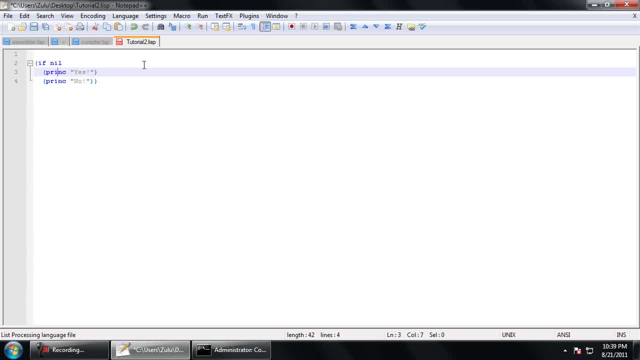 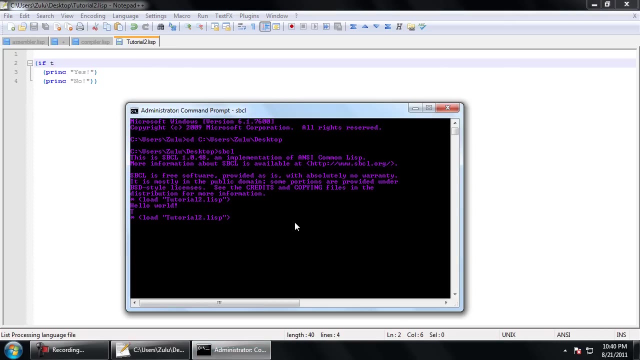 if it is nil. if this instead was nil, it's going to evaluate the second argument or that, the third argument, the, the else. so if we go ahead and type, let's leave that as that, go back to SBCL and let's load that file up again. 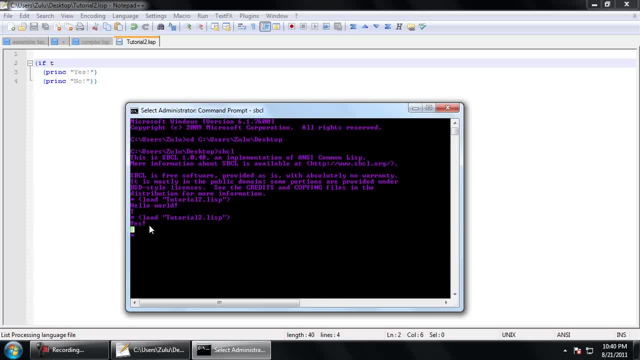 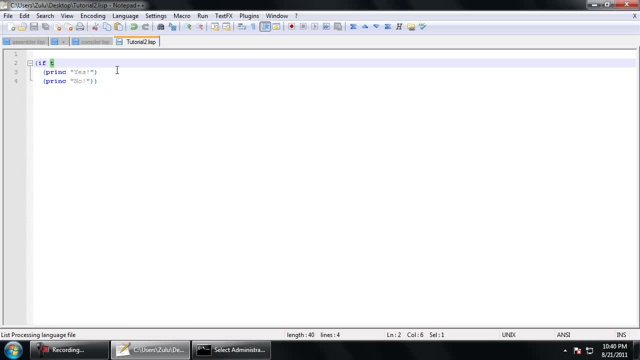 you can see that we have the output of yes and again the T from from load. the yes was produced because the if saw this return, the value T. it saw that it's not nil, so I went ahead and executed this if this had been nil, as we'll see now, it's going to instead evaluate this. 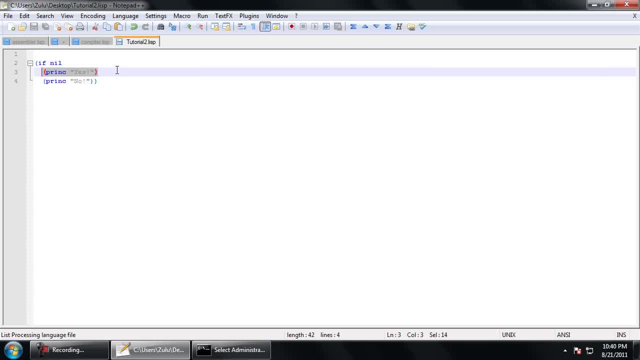 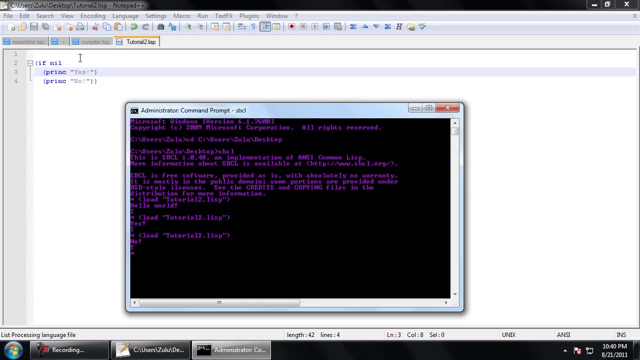 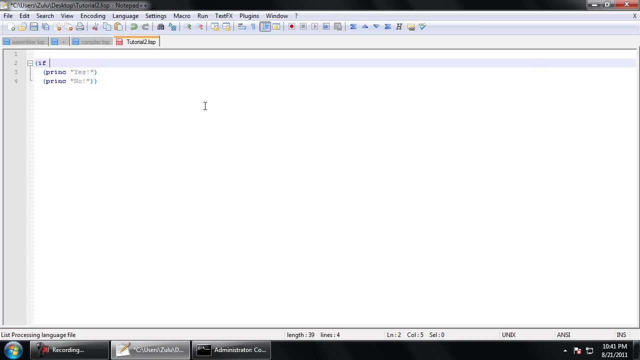 without evaluating this, this, this will, this very. the second argument is only evaluated with the truth value here, so let's have it like this and see what that produces. no, which is correct as per my definition or my description, and just to show that anything is true other than nil, we can put here a 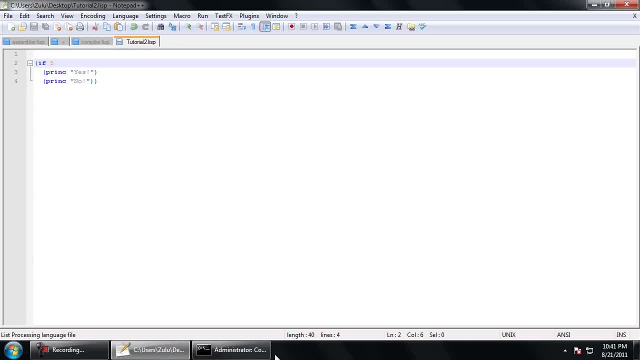 and just to show that anything is true other than nil, we can put here a, for example, five. this is a random number. for example, five, this is a random number. for example, five, this is a random number. and let's go and load that and we see, we. 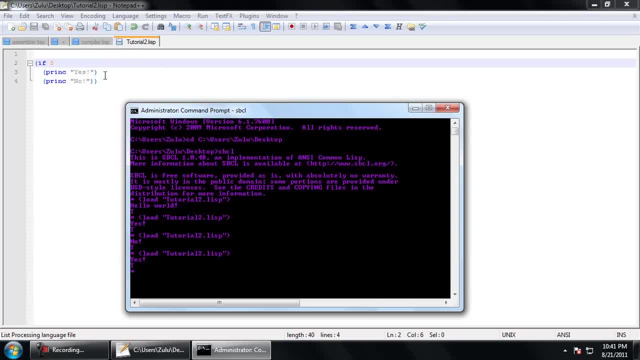 and let's go and load that. and we see, we, and let's go and load that, and we see we have the output of yes produced also, have the output of yes produced also, have the output of yes produced also for you. see, you guys out there, if I put 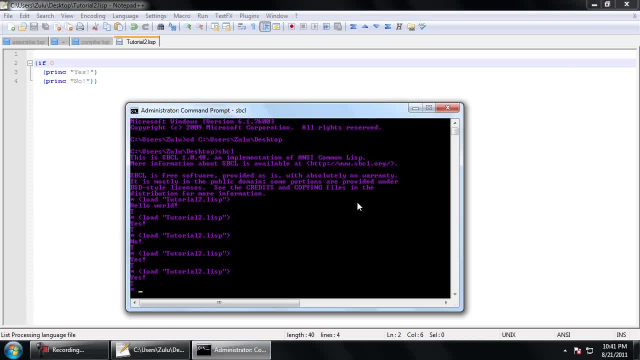 for you. see you guys out there. if I put: for you, see you guys out there. if I put: if zero it's still true, this is because if zero it's still true. this is because if zero it's still true. this is because zero is not the same as no. nil is a.